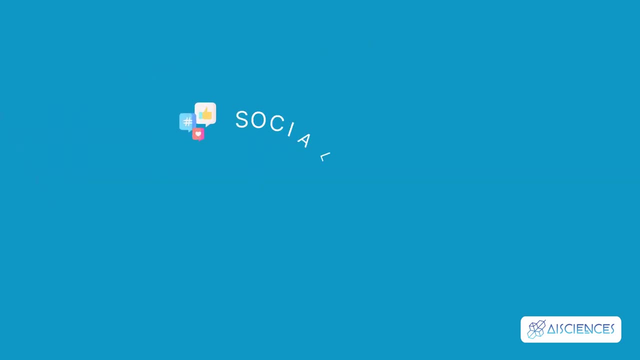 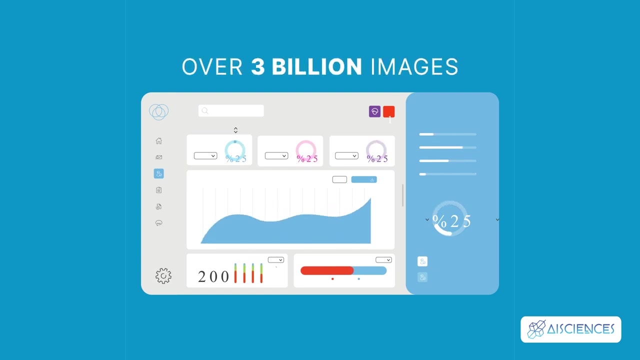 Images dominate the Internet today. They are everywhere: Social media, e-commerce stores, travel sites and more- But along with an enormous amount of visual data. over three billion images are shared every day. But along with an enormous amount of visual data: over three billion images are shared every day. 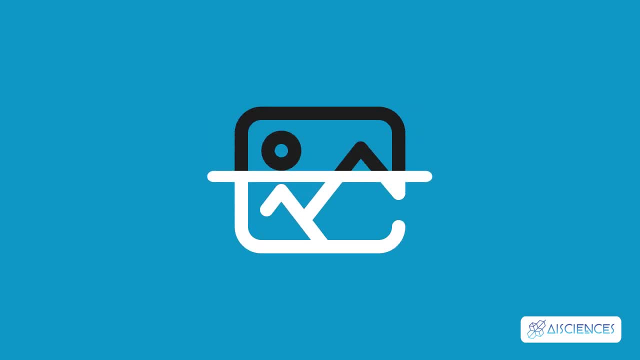 We also have easy access to the computing power needed to analyze this data. We also have easy access to the computing power needed to analyze this data. Computer vision is a booming field. Computer vision is a booming field. the latest advancements in this field. It's true that the field of computer vision has grown. 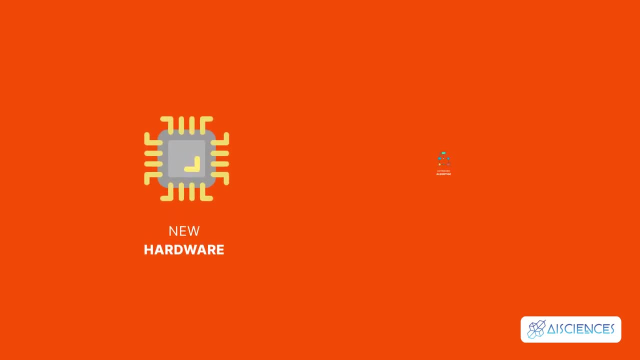 exponentially in the last few years alone. New hardware and advanced algorithms have ensured that the accuracy rates for object identification are high. In less than a decade, the improvement in the accuracy percentage has been phenomenal. It's gone up from 50% to 99%, making today's 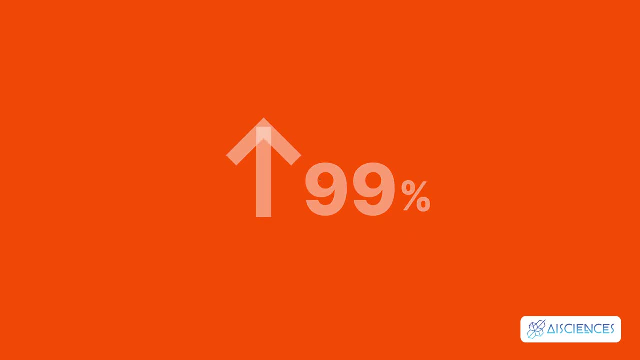 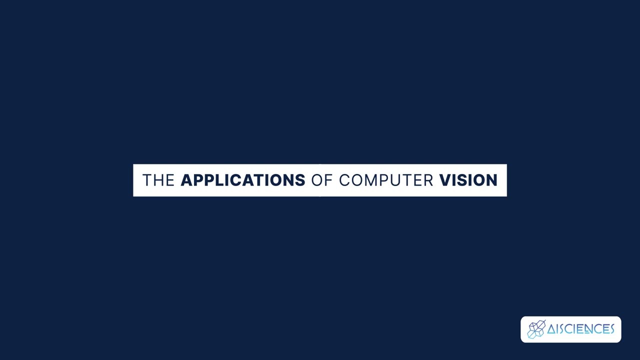 systems more accurate than humans. It's an accepted fact that computers react much more quickly than humans to visual inputs. The Applications of Computer Vision: The earliest experiments in computer vision began in the 1950s. Computer vision was, however, first put to commercial use only in the 1970s to differentiate typed text from handwritten text. 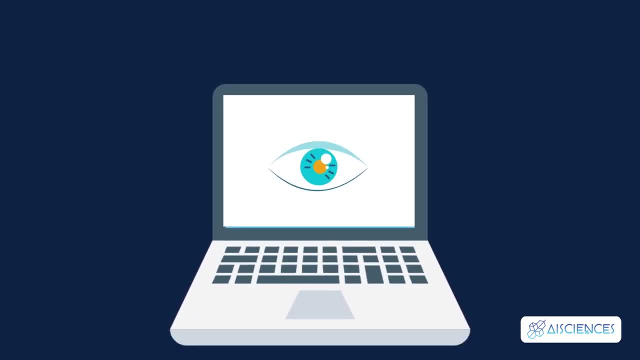 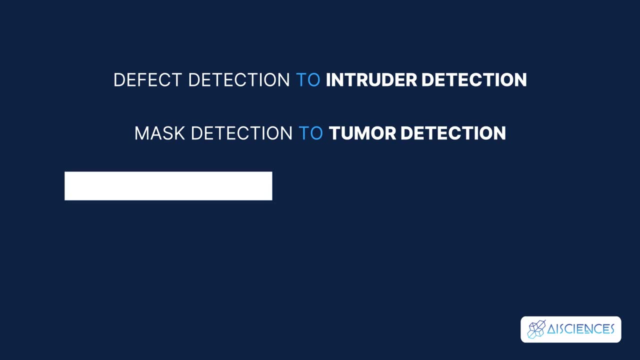 But today computer vision is a reliable and mature technology that generates huge cost savings and saves time: From defect detection to intruder detection, mask detection to tumor detection, crop monitoring to plant monitoring, vehicle classification to traffic flow analysis, and from customer tracking to theft detection. 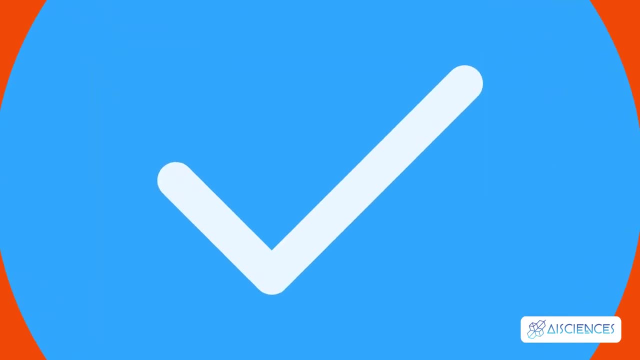 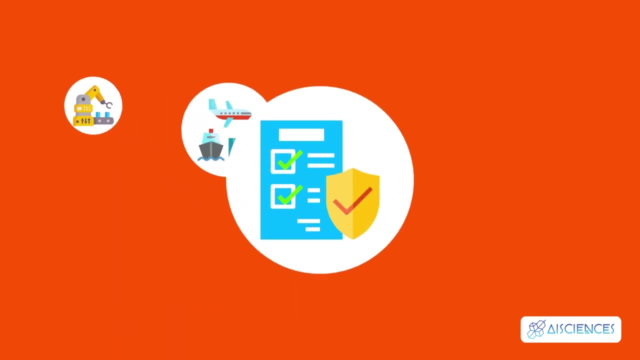 the applications of computer vision are truly varied. Computer vision is used extensively in the following fields: Retail & manufacturing, Transportation, Insurance, Media, Agriculture, Health Care, Sports, Banking, Augmented Reality & Mixed Reality, Home Security, and Content Management and Analysis. 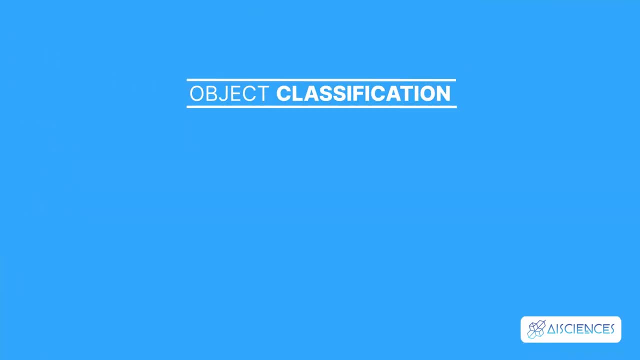 The most powerful and most highly reliable information in the market is the field of you To make ideas. Most popular computer vision applications include: Object Classification: recognizing the broad category of an object in a photograph. Object Identification: identifying the type of object in a photograph. Object Detection: detecting the location of.